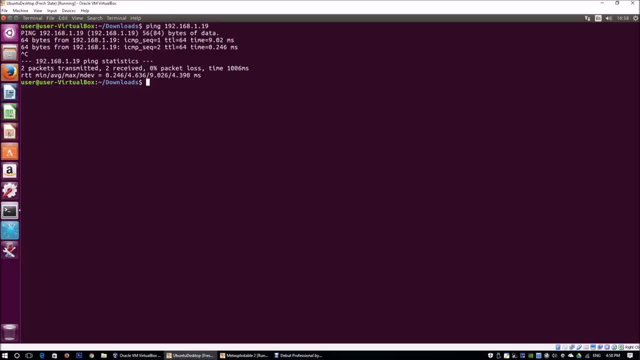 So on the background, I have Ubuntu running. So Ubuntu is going to help us Surf the attack using LLIC and we will be able to cut our attacks and this will be able to prevent any kind of attacks that are possible, And it's going to be a lot of fun. 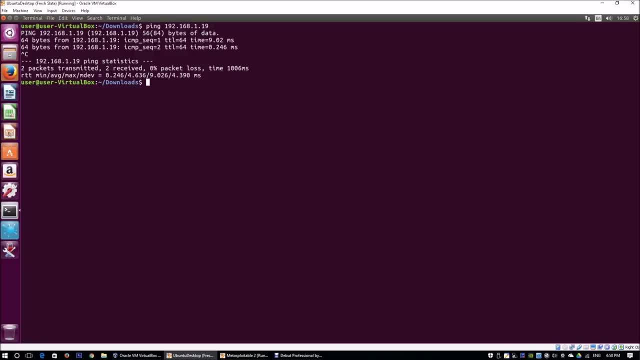 And at the same time, we're going to use Wireshark as a network protocol analyzer to really study about how the whole idea of connecting between the transport layer and to understand how this denial of service actually works. So what's going to happen over here is I'm going to enter sudo wireshark. 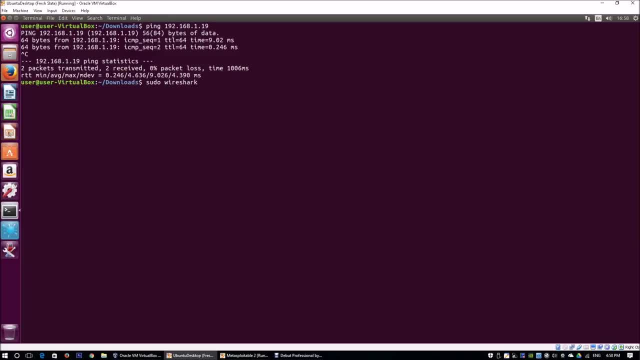 So this will help launch Wireshark in my virtual machine. So enter sudo. So of course it's asking for your password, So you just enter the password that is required for you to authenticate And to use the super user. So now I have Wireshark running. 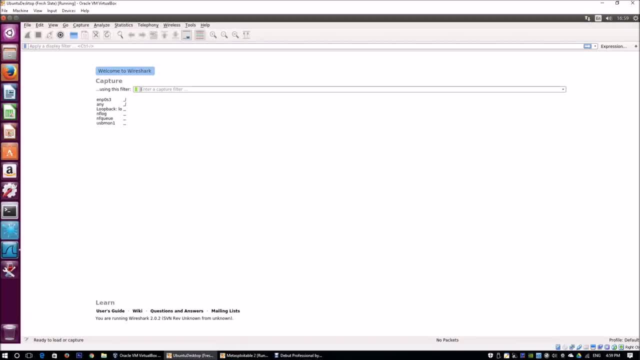 Of course it's already running And I can see that I have a few network interfaces that I can use. So of course I'm going to use the first one, which is EMP0S3.. So you double click on it. 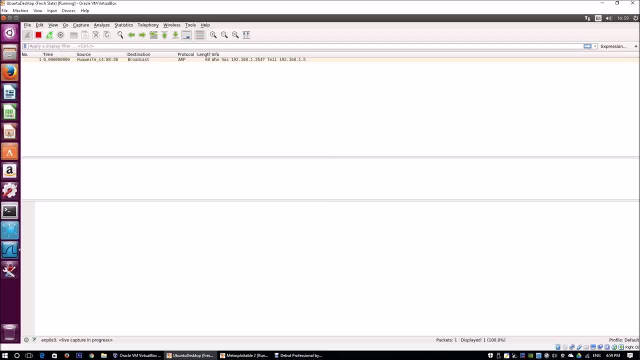 And it's going to open up the network protocol analyzer That's going to check against this network interface. So of course over here I can see this is actually one of my phones that is running on the network that's trying to ask for. 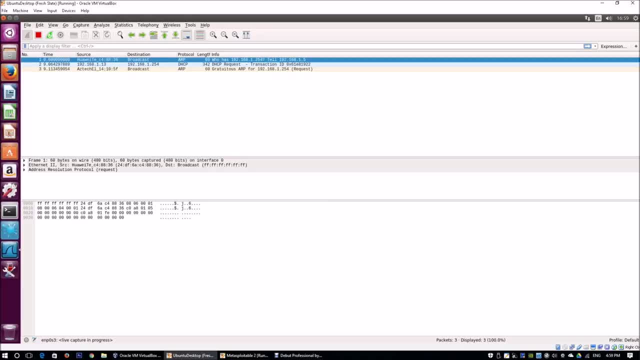 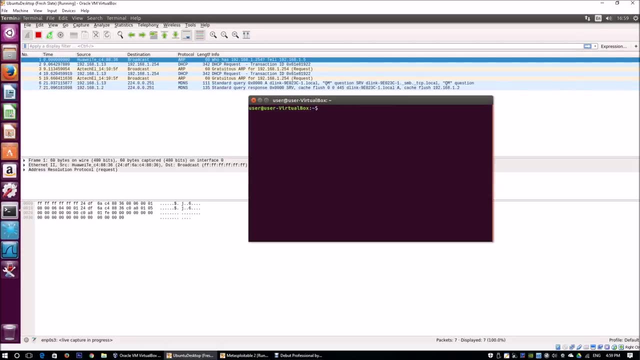 the network protocol analyzer. Where is who is 192.168.1.254.. So, of course, going back to the terminal, going back to the terminal over here, what I'm going to do is I'm going to launch the LOIC. 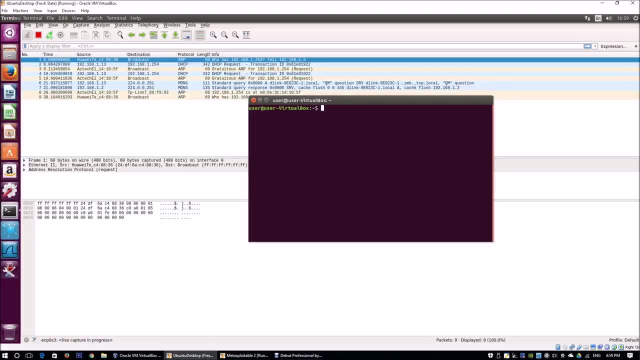 So low orbit ion cannon is going to help us do some conduct some denial of service attacks by flooding it with a lot of network traffic. So all you got to do is enter mono. So I got to go to download first. So I have already downloaded LOICexe. 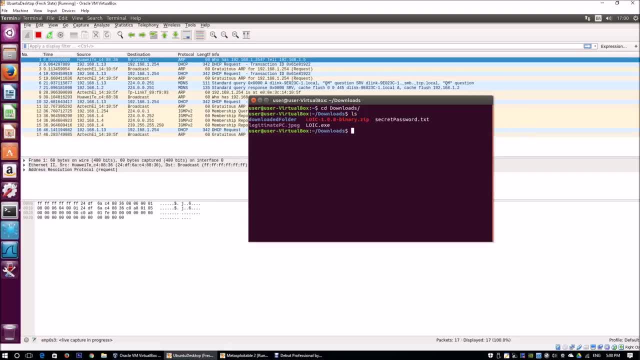 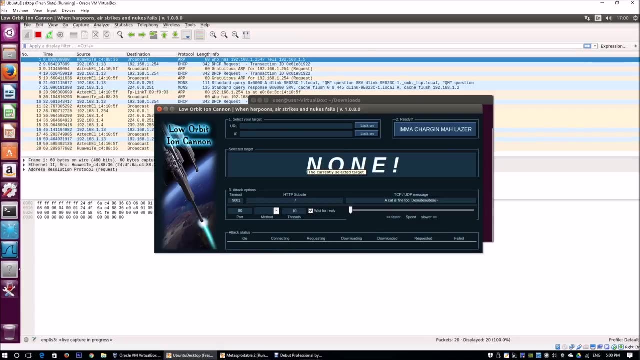 So what we're going to do is we're going to launch it so you can enter mono and then followed by LOICexe, So this will actually launch LOIC. So over here we have low orbit ion cannon. So what's going to happen is that you're going to enter the IP address first. 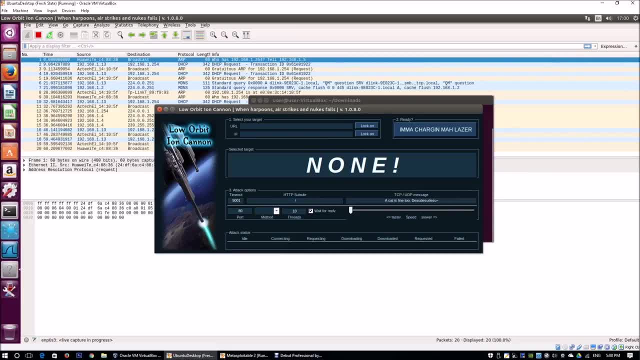 So, remember, the IP address is 182.168.1.19.. And, of course, over here on the number three, on the attack options. So we're going to use port 80.. And do you want to use transport control protocol? 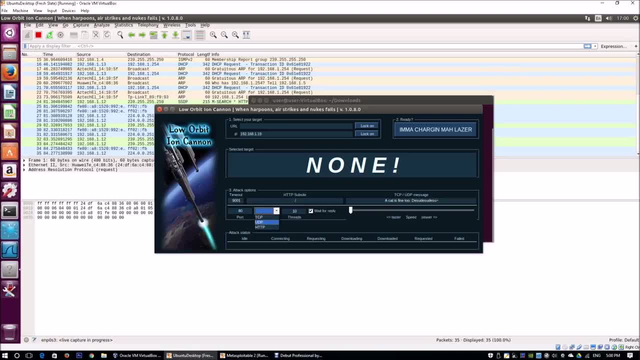 Or do you want to use user data diagram protocol? So we're going to use UDP And of course, we're not going to wait for reply, And with this we have 10 threats. So what's going to happen is that we're 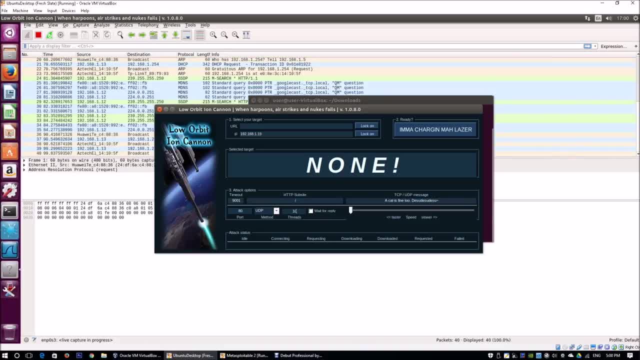 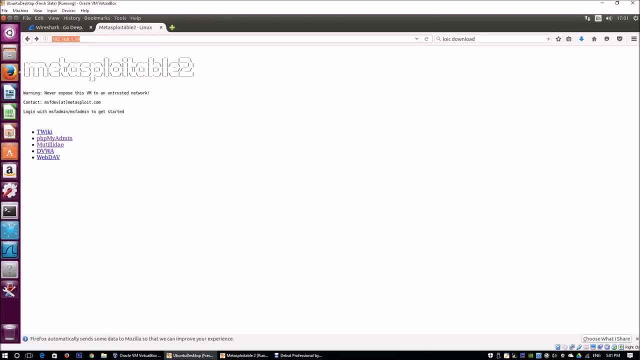 going to send a lot of network traffic requests to the web server And the whole point of denial of service is to flood it with so much requests That he has no time to actually respond to legitimate or authentic requests coming into the server. So when I go back to Firefox and I enter 182.168.1.19,. 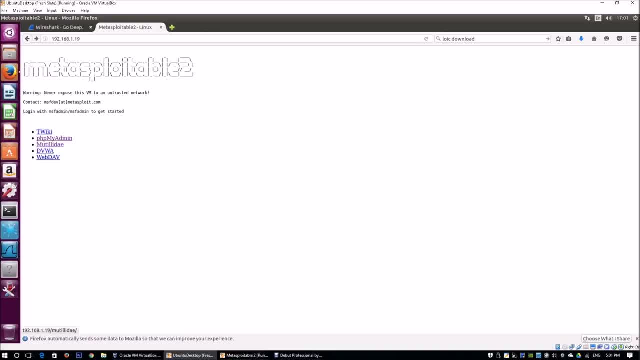 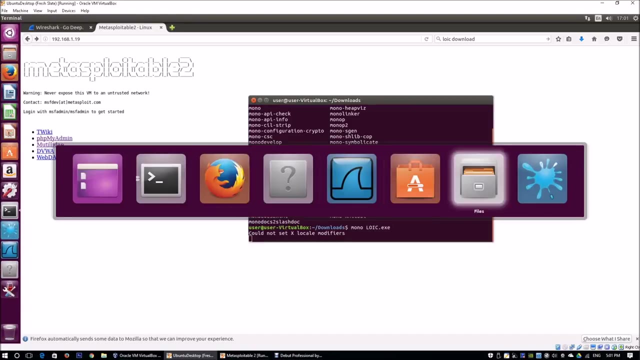 I'm actually able to access the services on the web server, So I can go to Mutiladay. I can go to phpMyAdmin. I'm able to access the site as intended. However, the point of the intrusion is actually for us to be able to attack. 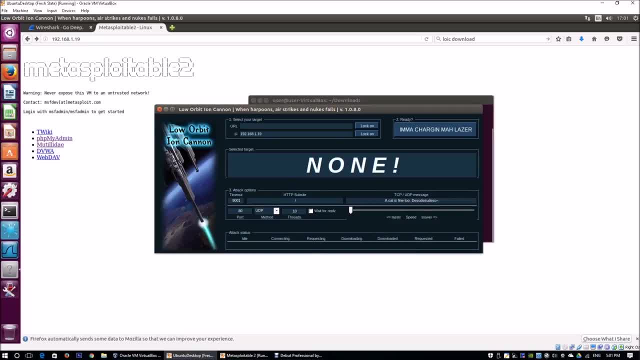 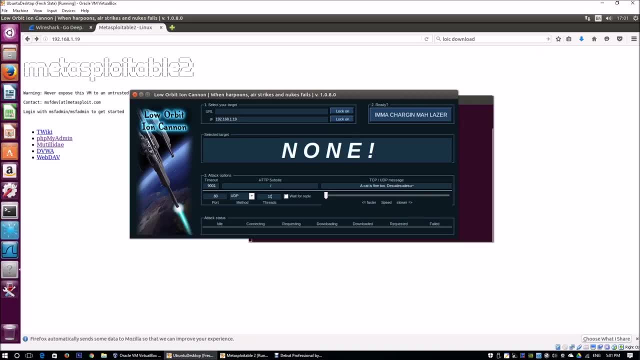 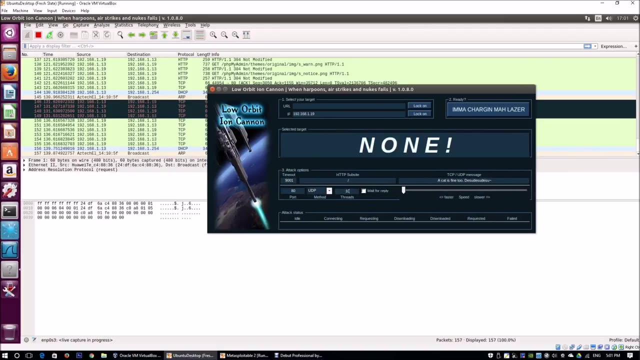 the system So that we may be able to override with so much requirements of resources, of computing resources, that a server can no longer respond to any other authentic requests. So going back to low orbit Ion Cannon. So what we're going to do is we have 10 threats over here and we're going to send 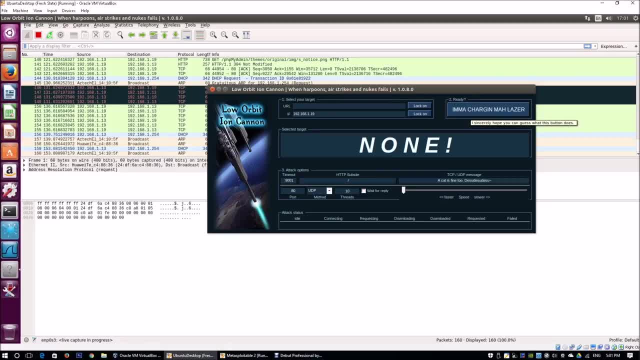 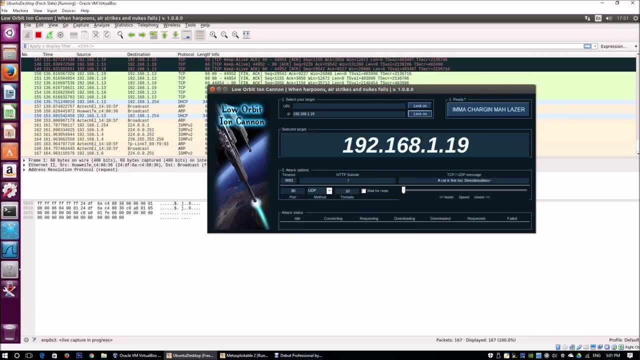 UDP requests and all you got to do is click on the. I'm a charging my laser, So you just click, click on it and, Oh, you got to lock in the, the attack first, 182.168.1.19, and click on the launch attack. 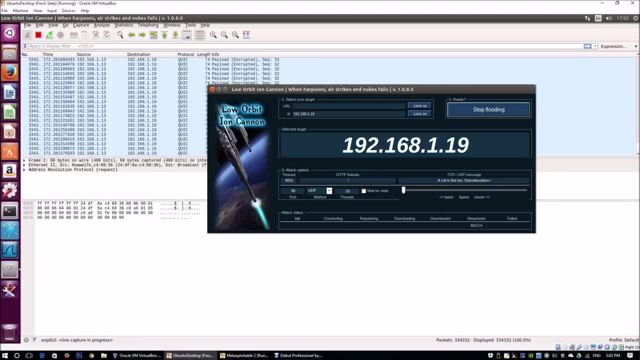 So it's going to start flooding. You see there's a lot of requested being sent over so I can click stop flooding. So the idea is that imagine you have multiple computers, you can launch multiple threats, maybe even 20 threats. You have a lot of processing power. 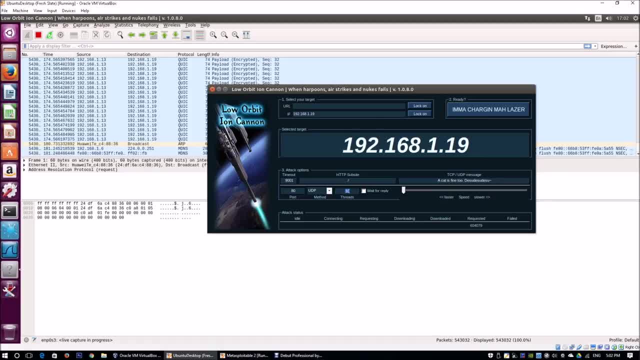 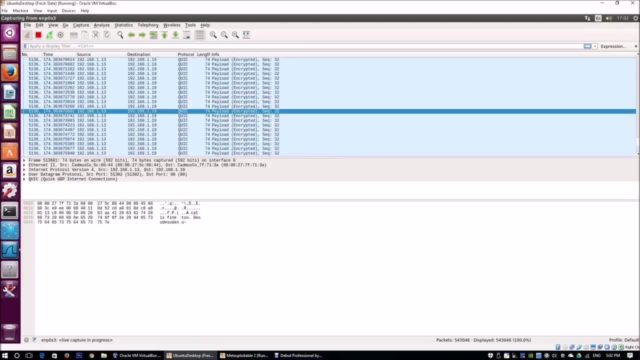 You can keep sending this information over using multiple computers into the web server And over here. if you look at Wireshark, you can see that we have the payload over here, So a cat is fine too, et cetera. 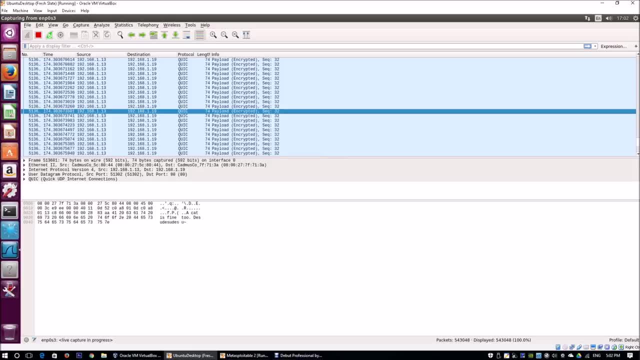 So all these are the information that is being sent over to the victim machine so we can overload the machine, so much so, until it's no longer able to respond to legitimate sites. So the whole goal is to keep sending plenty of this information over and to be able to flood it with so much requests that it 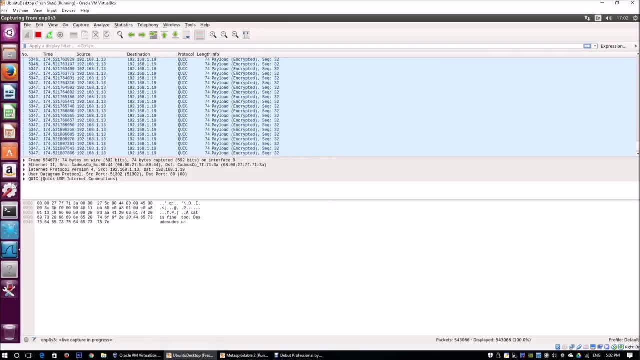 can no longer function properly. So this is how denial of service attacks actually work using LOIC. So, additionally, you can increase the number of threats. You can change the transport layer protocol to TCP, So it's going to be having different results, as a TCP requires three-way handshake to complete the connection. 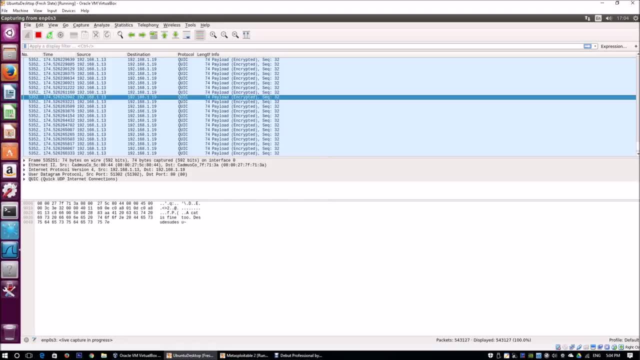 And, of course, UDP is a fire way to be able to flood the information onto the web server. So all these are techniques that you can actually use on low upbeat on Canon. you can download it from the site and you'll be able to launch it on Windows machine. 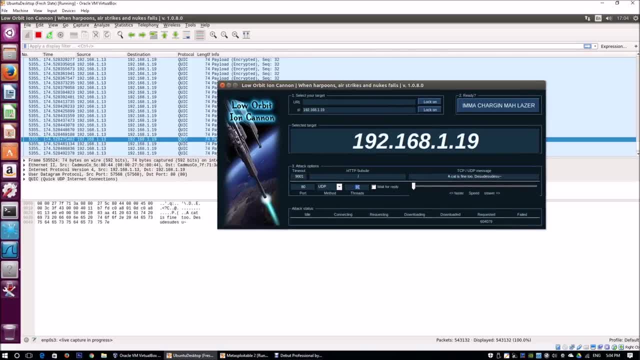 So over here I'm actually using Mono to run it as an exe file And of course you can change the attack to TCP. So if we look over here on the latest, latest network traffic, we can change it to TCP as well. 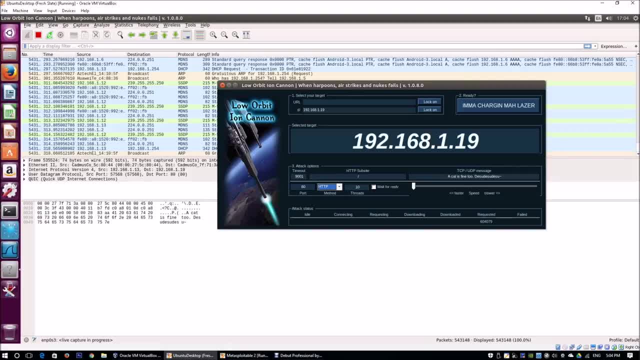 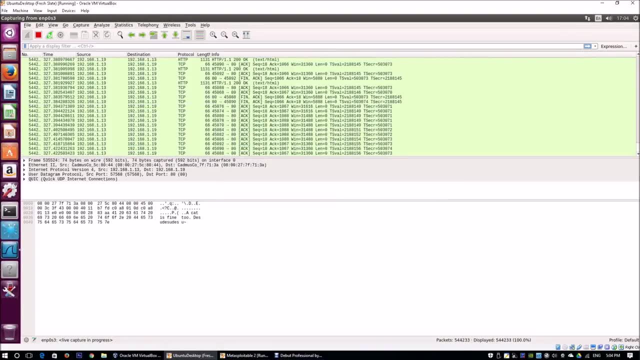 And of course, we can launch the attack, or we can change the HTTP And, of course- same thing- we can launch the attack as well. So if you see over here, I'm going to click stop flooding. So what you're going to see is that we have sent a lot. 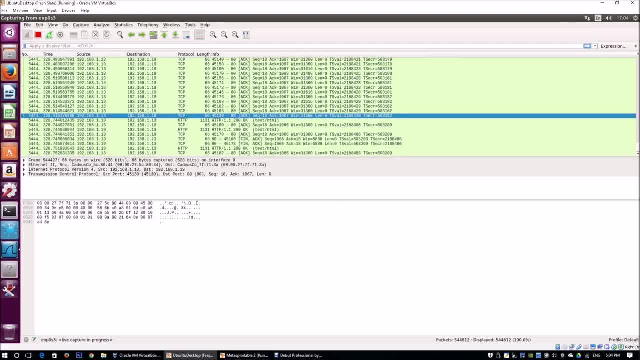 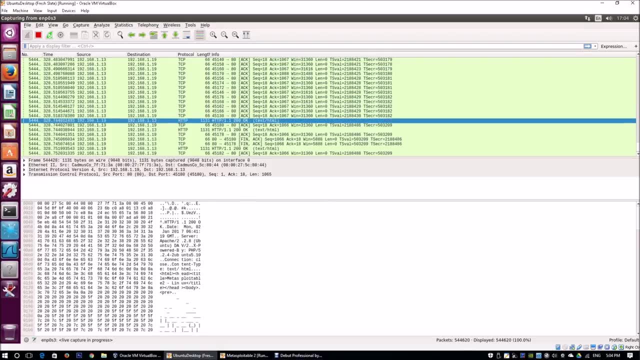 of information over to the IP address, and what's happening is that you can see the source as 192.168.1.1.3 to the destination of 192.168.1.1.9.. And what's happening over here is that you. 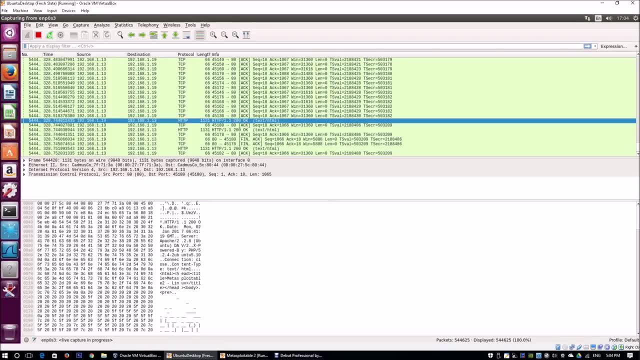 see a return address or return information from the web server to you. So it actually consumes computing resources from the web server. So even multiple attacks of this is going to take up a lot of computing resources from the web server And what's going to happen is going. 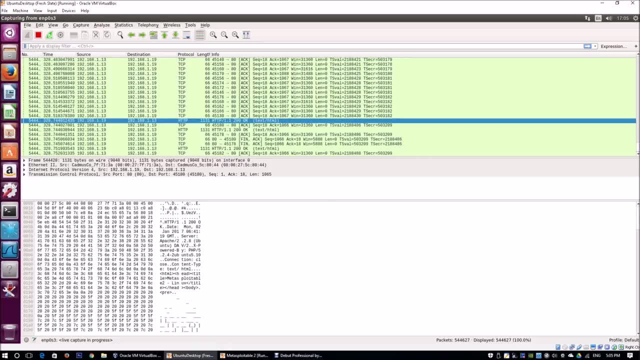 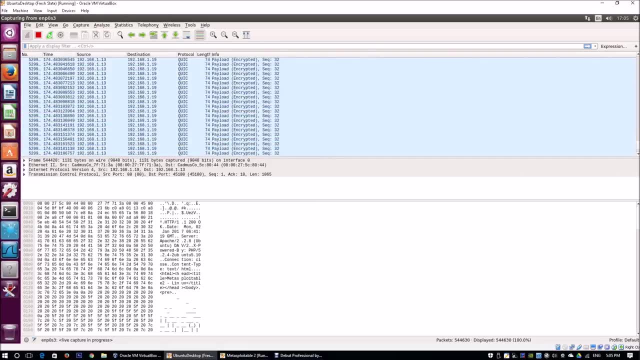 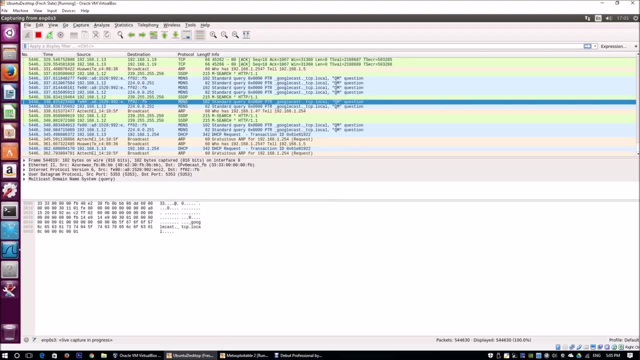 to delay the responses to legitimate and authentic requests coming from the users. So you as a, as a hacker, the whole idea is: what can I do to to increase the number of requests? and if you are a web developer or web administrator, then the question is: is there anything you can do to filter off all? 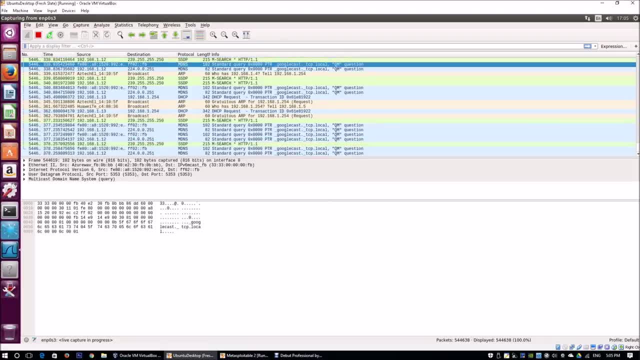 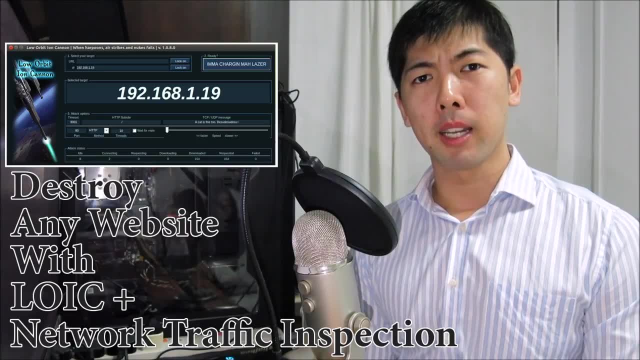 these attacks that are illegitimate, that are malicious in nature? What can I do to filter them away? So you've seen how easy it was in the demonstration to actually provide a flood using the LOIC tool and spec the network traffic coming from LOIC to the web server. 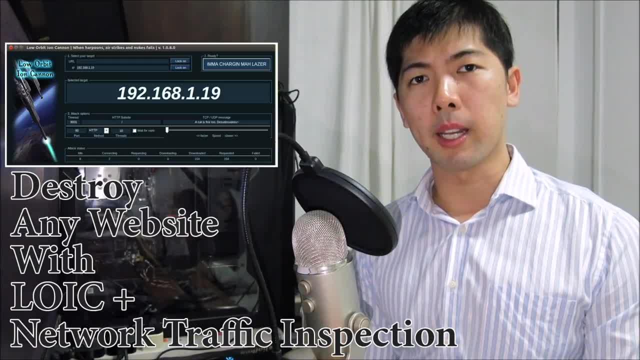 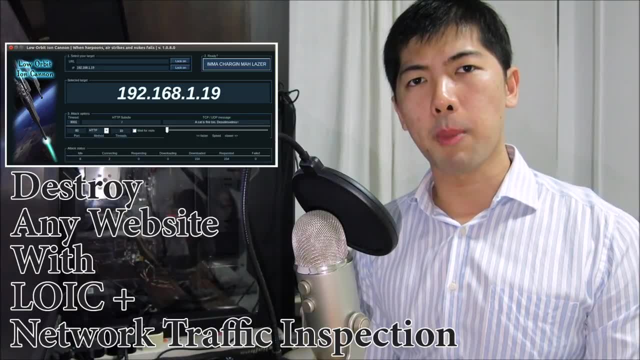 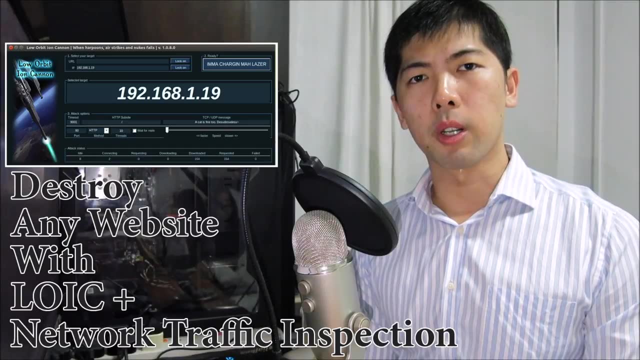 And from there you understand exactly how we can actually flood the web server with a lot of illegitimate requests, malicious requests, and overwhelm the web server from responding to legitimate requests. So the idea is pretty simple, And the greater part is that, if you were, 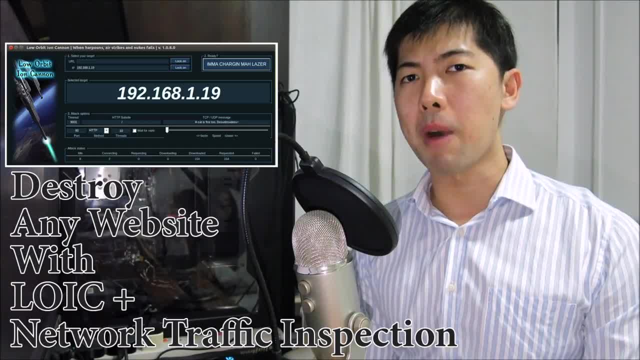 to perform a distributed denial of service attack. you could install multiple LOIC and tens of thousands, even hundreds of thousands of devices and you could push the UDP, TCP or even HTTP flooding over into the web server, and that would actually take down a lot of massive servers around the world. 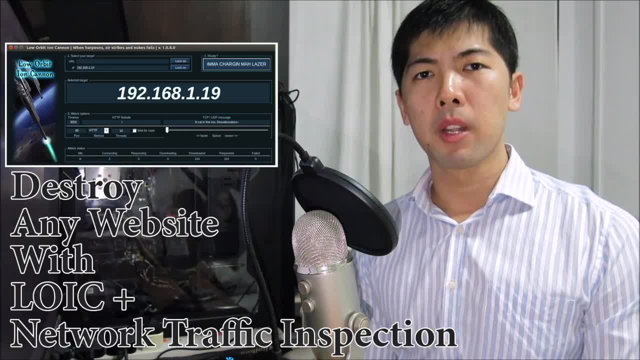 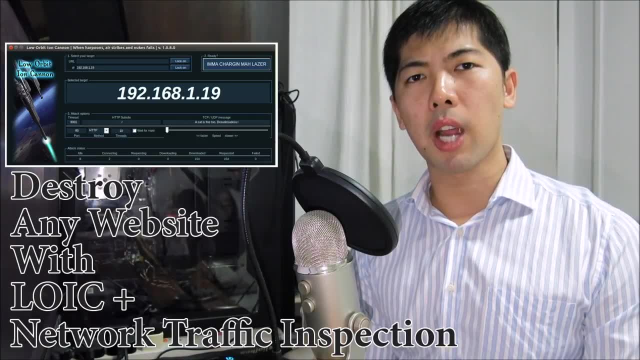 So I think some of the hacking incidents that happened in 2016, there were huge distributed denial of service attacks coming from Internet of Things devices And what happened was that it shut down the entire servers- domain servers- from actually being able to respond properly to those requests. 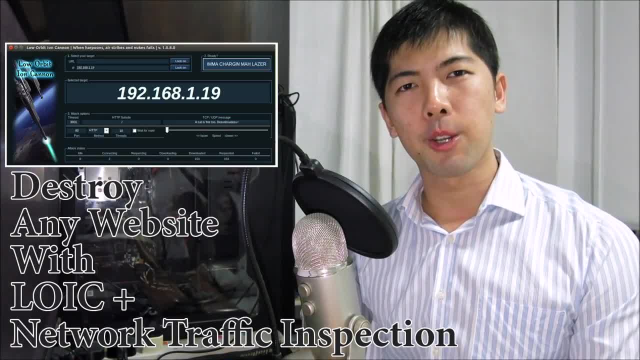 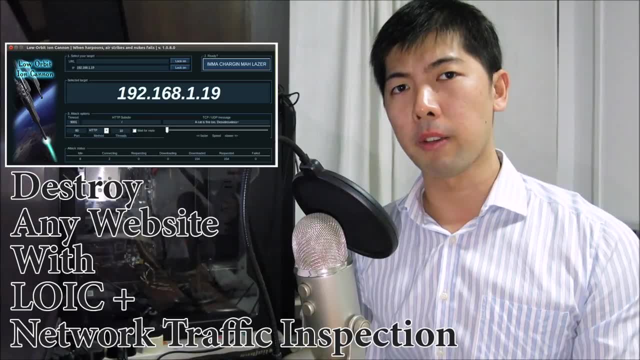 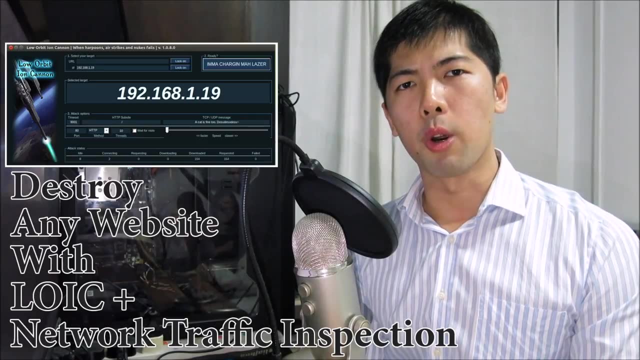 So, moving forward, the question will be: how can we defend against such denial of service attacks? So one of the really easy ways is to use web application firewall or to have simple firewall configurations like filtering of certain IP addresses, blacklisted IP addresses, or to filter against a massive sending. 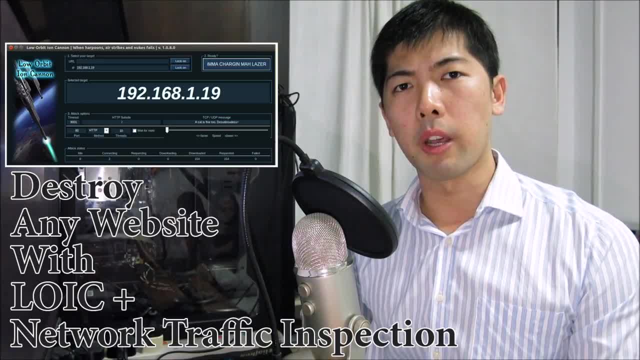 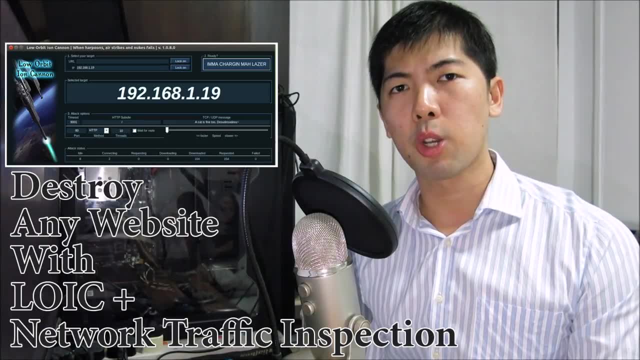 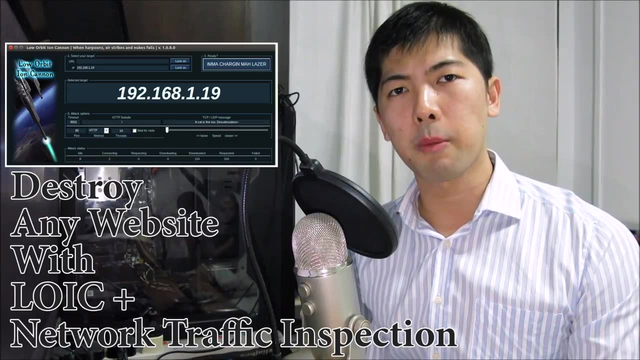 of network traffic from a particular source. So if a source were to send like 10 times the amount of UDP packets or TCP packets per second, and then chances are it could be a malicious activity coming to attack your web server and all you got to do is just discard that packet. 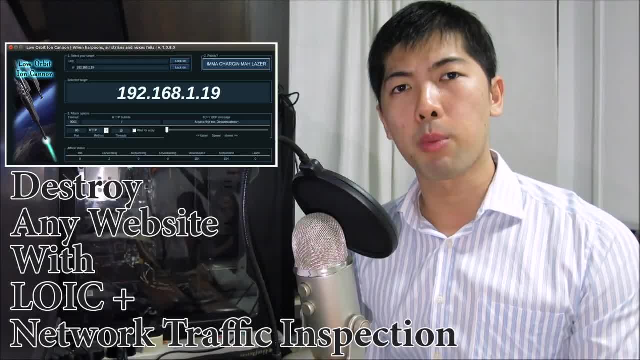 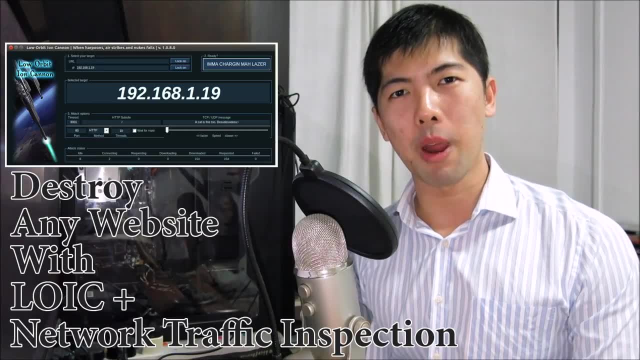 look through the packet using a firewall, discard it, and you'll be able to respond properly to legitimate requests, though that can be one way of defending your web servers And, of course, in conjunction with web application firewall or firewall, you can actually use distributed network. 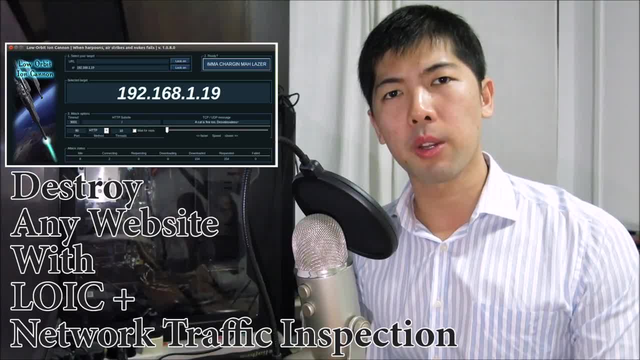 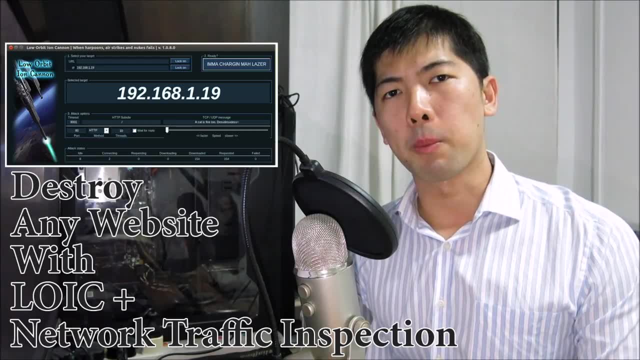 or load balancers to be able to distribute the requests coming from different kind of sites. So, after, perhaps, your firewall has filtered the requests, you have multiple servers around the world, you have different data centers around the sites and you'll be able to distribute the content or the flooding. 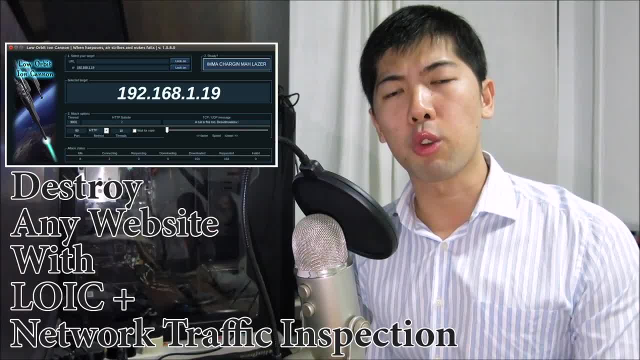 of attack coming in from one server to others And you'll be able to distribute the resources, the computing resources, and be able to alert the administrators on some of the malicious activities. And if there's a spike in a network traffic, you'll be able to take it down, blacklist the IP address again or to disable certain.